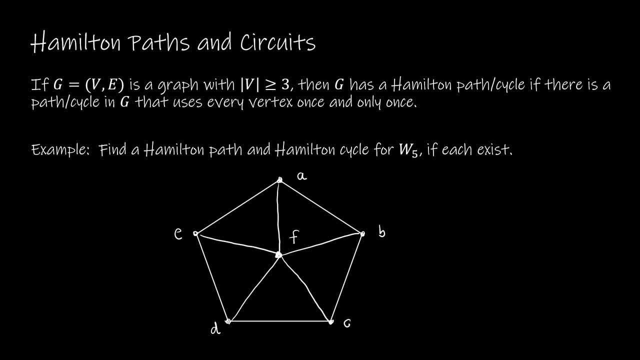 once and then travel back to our beginning vertex. So, even though we say that it uses each vertex once and only once, if we're talking about a circuit, we will begin and end at the same vertex. For a path, we don't begin and end at the same vertex, but we still visit every vertex. 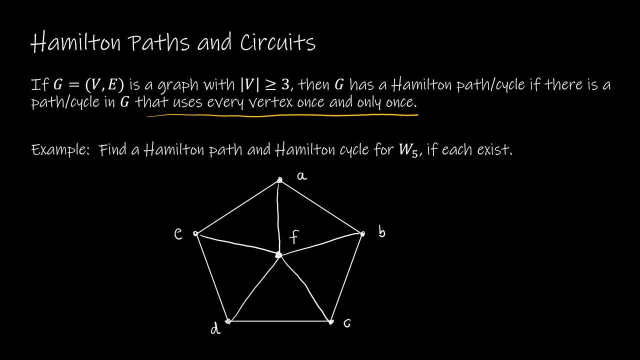 So, for instance, see if we can find a Hamilton circuit, Hamilton path and a Hamilton cycle for W5, so the wheel graph, if each exists. So if I start, say, at A, I want to visit every vertex once and only once, and end up back at A. 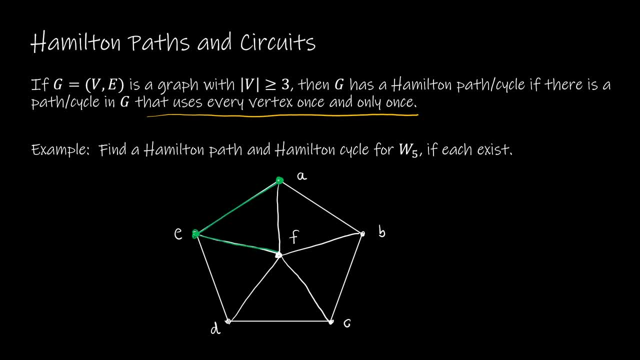 So let's say I travel to E, then to F, then to D, then to C, then to B, then to A. So I went A, E, F, D, C, B, A. That is a Hamilton cycle. So what's a Hamilton path? 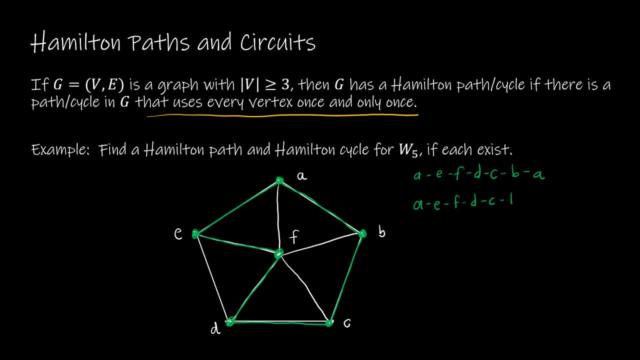 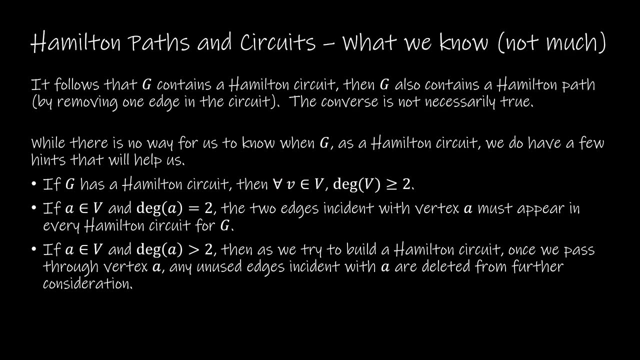 A, E, F, D, C, B, So I just don't finish and go back to A. Now it would be great if there was some algorithm that told us exactly whether or not there was a Hamilton path or circuit or how to find it. But unfortunately, 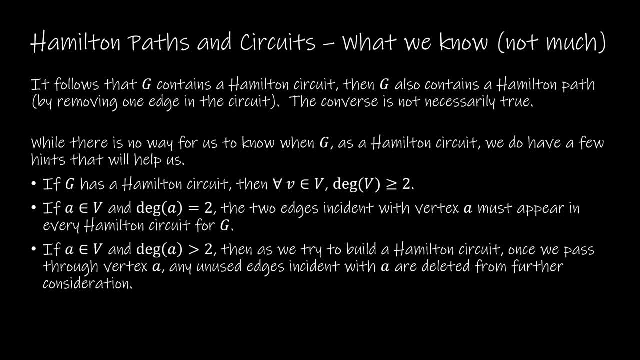 that does not exist for Hamilton paths or circuits. So all we can do is take a look at what we know is true and then basically just give it a shot. So here's what we know about Hamilton paths and circuits. So if G contains a Hamilton circuit, then G also contains a Hamilton path, by simply. 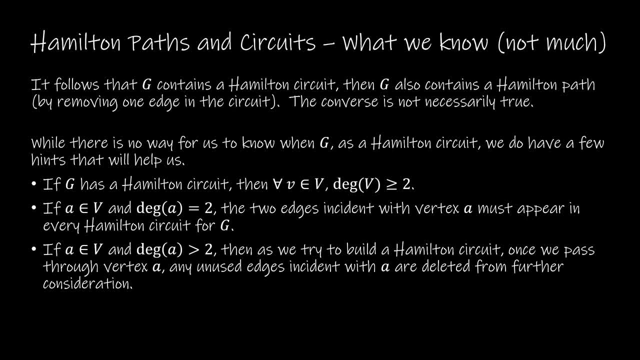 taking away that last edge which we just talked about on our last example. But of course the converse is not necessarily true. Now again, there's no form for us to know when there is a Hamilton circuit, but we do have a few hints that will help us. So if G has a Hamilton circuit, 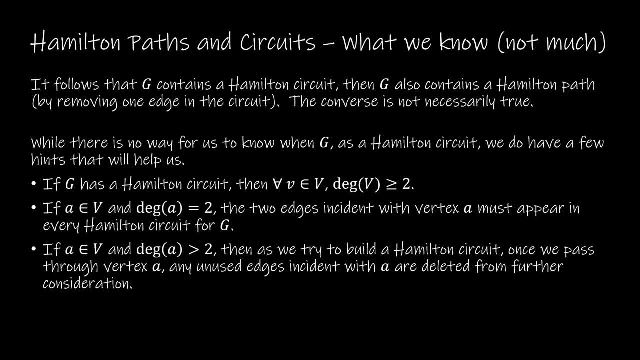 then each vertex has degree of at least two. So right away, if we look at a graph and we have a vertex of degree one, it's not going to have a circuit. Now it could have a path, but it's not going to have a circuit because again we would have to end up. beginning to have a path. So if G has a Hamilton circuit, then each vertex has degree of at least two. So if G has a Hamilton circuit, then each vertex has degree of at least two. So if G has a Hamilton circuit, then each vertex has degree of at least two. So if G has a Hamilton circuit,